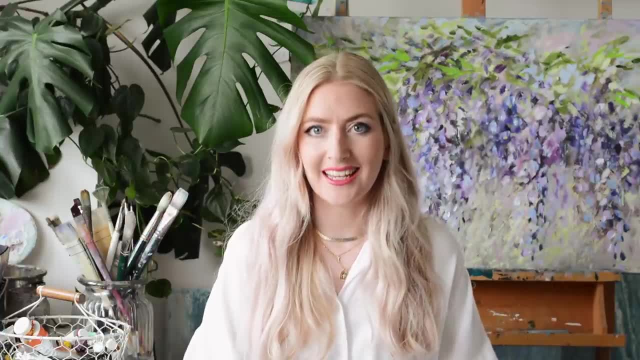 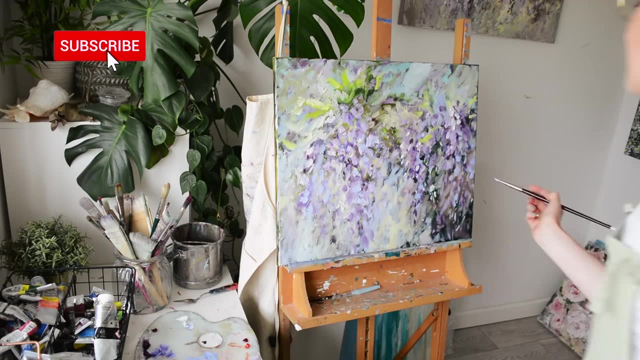 Hi guys, and welcome to 10 tips to paint impressionistic. I know a lot of you really want to paint impressionistic but really struggle and end up making your painting too detailed, and so today I want to give you some tips on how you can paint in an impressionistic way. So tip one: 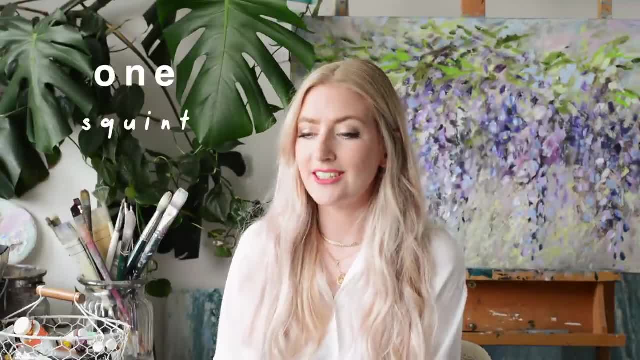 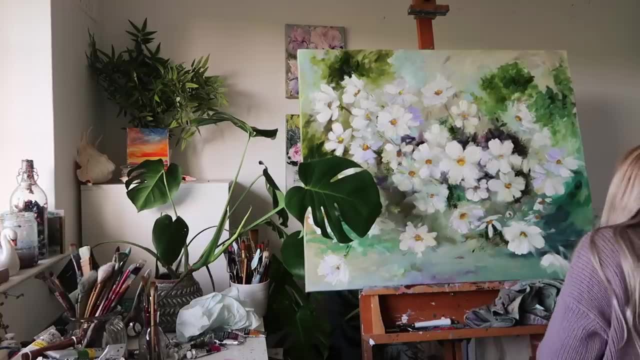 is to squint at your painting. I know it sounds a bit strange and, yes, you might look a bit silly, like I do in my videos, but if you squint it really helps you to block out all the unnecessary data and just focus on the proper value composition, which is what you need when 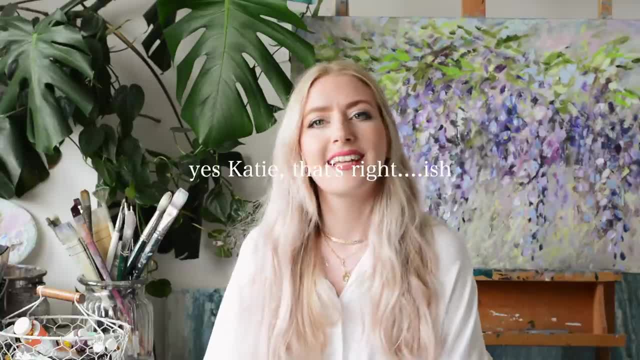 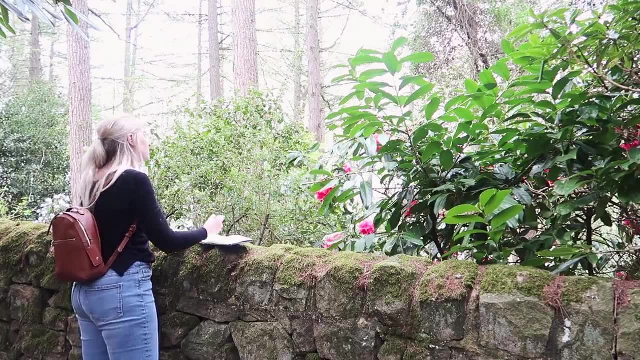 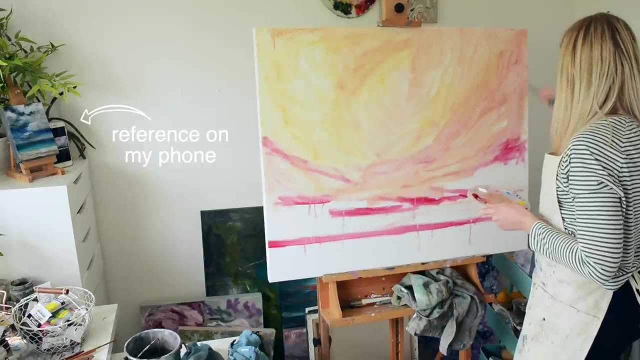 you're painting an impressionistic painting, Wait. Tip two: use a reference photo and keep it far away. So if you're using a real life reference, then you might need to squint at that as well, but if you're using a photo on a device like an iPad or a phone, or a real life photo, keep it a. 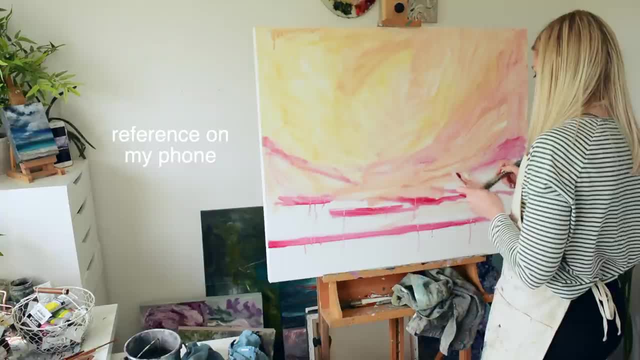 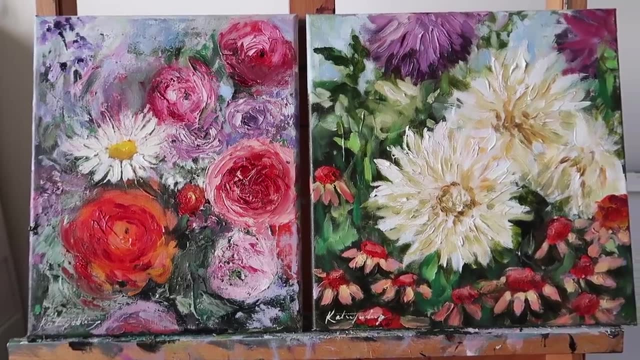 bit further away so you're not so caught up on the details. You just see the main body of what it is you want to capture and then you can let the paint be the details, Those little gorgeous nuggets of painting. they can be the details. Tip number three is: don't worry about 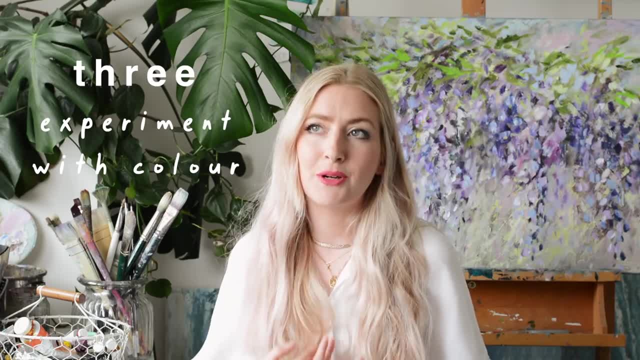 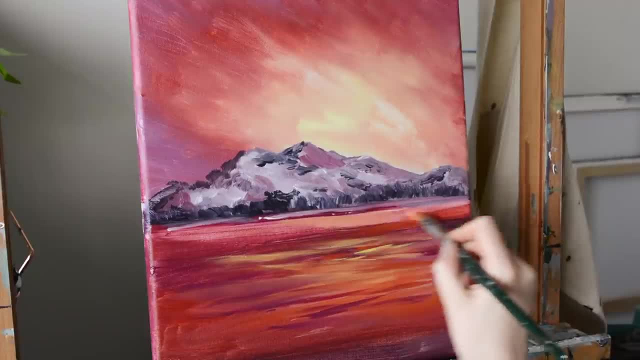 what the real life colours are. This is your moment to use your imagination, add in whatever colours you want, whether that's using all very similar colours, using opposite colours on the colour wheel. This is your time to experiment, and that is the fun part. Tip number four is to focus. on value, and if you're using a reference photo, then you want to keep that in mind. So if you're using a reference photo, then you want to keep that in mind. So if you're using a reference photo, then you want to keep that in mind. So if you're using a reference photo, then you want to keep that. 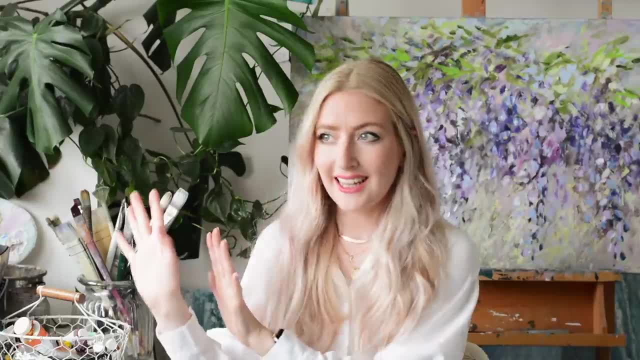 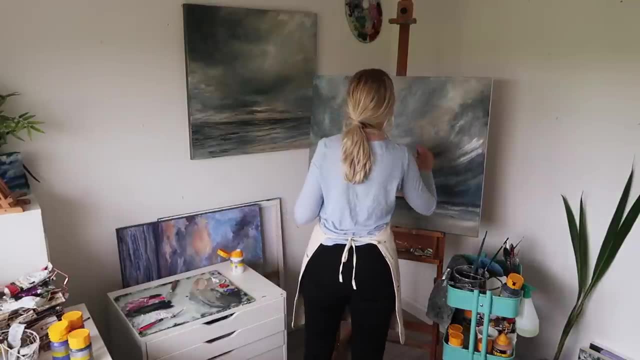 in mind. Tip number five is to use the intensity of colour so that your painting doesn't look messy. so if you're painting a landscape, the things in the distance still need to be lighter in colour and still need to be less intense in colour, with less saturation, so that it still has that realistic. 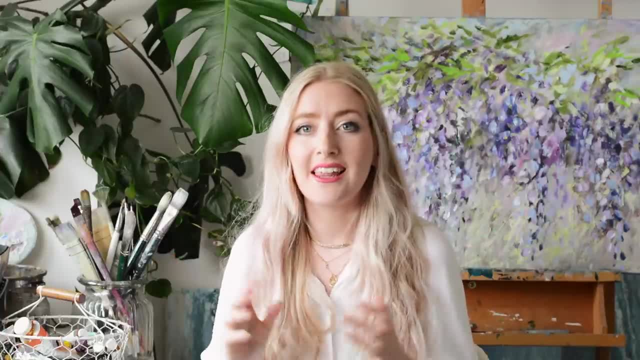 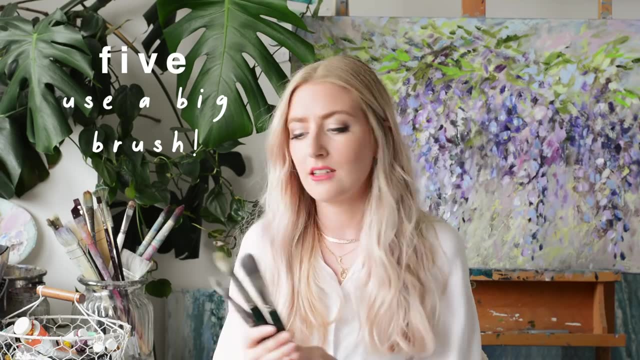 edge and it looks realistic, but in an impressionistic way, and that is one of the main tips to stop it looking like an amateur painting. Tip number five is to use a big brush. These are some of my favourite brushes, which, you can see, are not small in themselves. This will really help you. 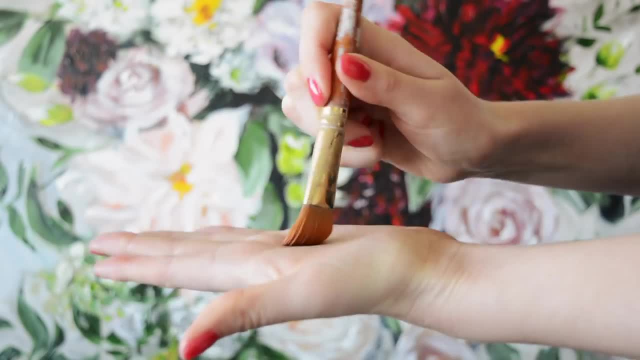 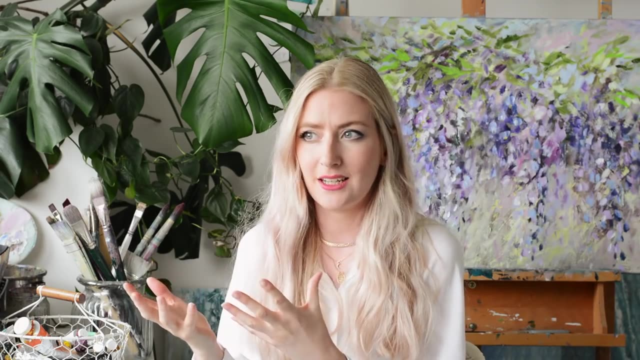 not focus on the details, but to add a big old brush stroke and let that do the talking. So that's one of my biggest tips: if you really end up making your painting look realistic- which you don't want to happen- and you end up focusing on details, which you don't want to do, Put away the 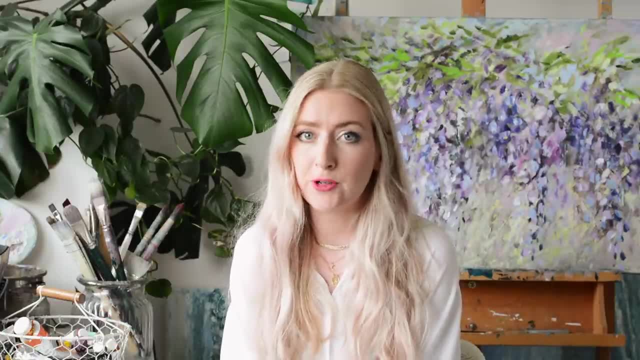 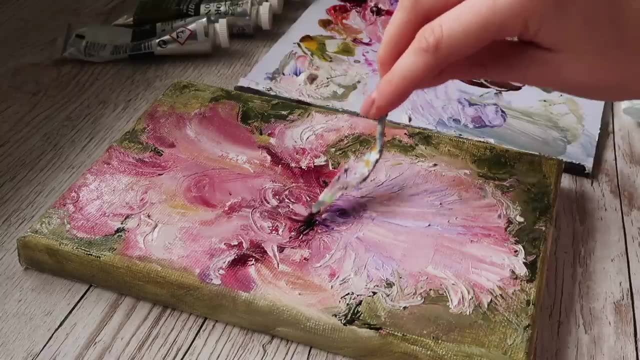 small paintbrushes, hide them and just focus on big brushes. Which leads me on to tip six, and that is to experiment with materials. So try using a palette knife or a rubber wedge. It might be difficult to do the whole painting like this, especially with the first few layers, but once 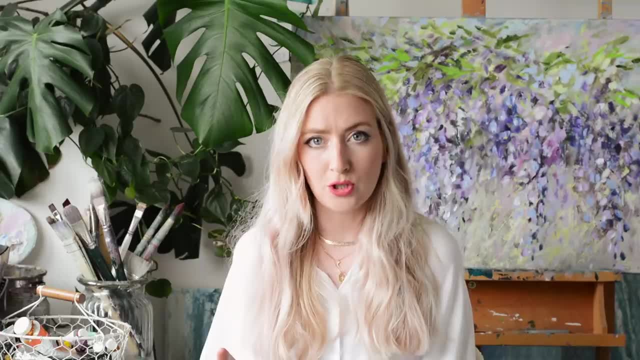 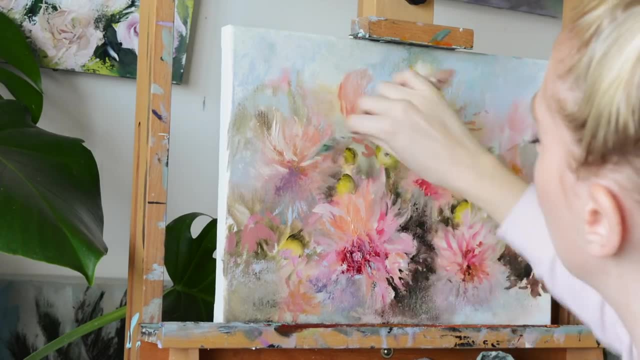 you've got the bulk of the painting, you can really use these different tools to give an impressionistic edge, and it really limits you so that you can't make it realistic, and that can be really helpful. Tip number seven is to hold the brush further down the handle. Sometimes we can. 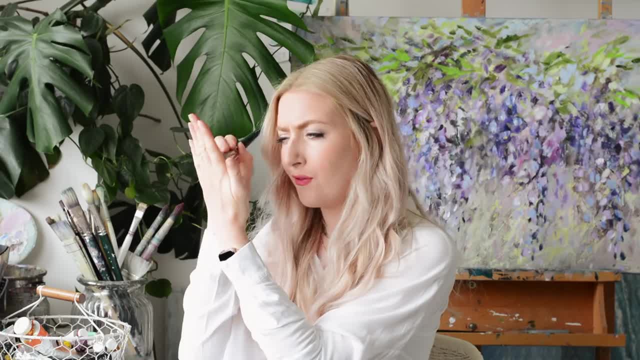 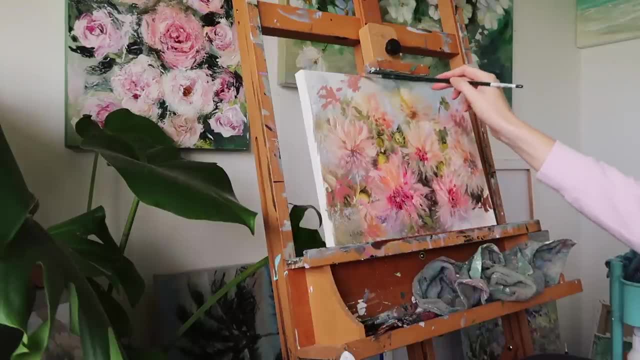 get so caught up in our painting that it's like here and we're focusing. Actually, it's much better to stand back, hold your brush further down the handle and sort of paint at a distance, and that will ultimately give you less control, which is what. 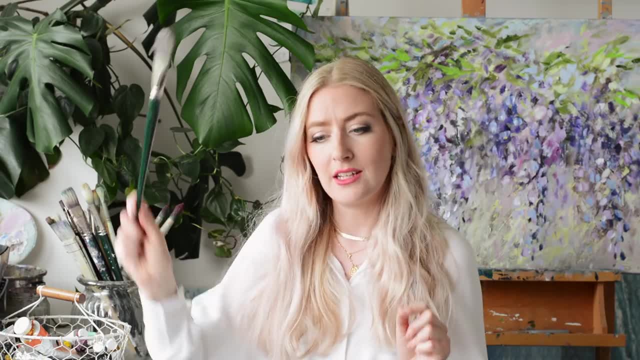 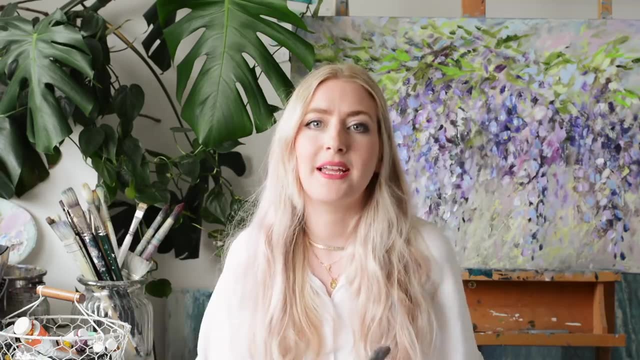 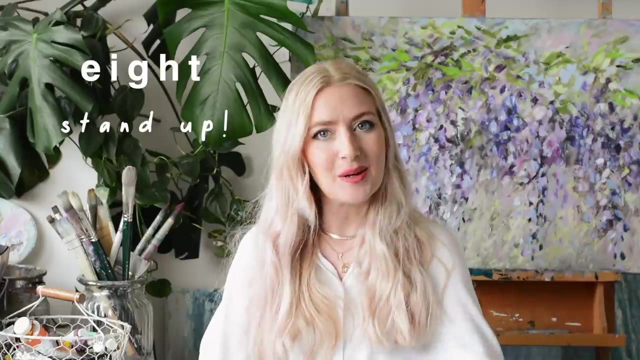 you want. but it also gives the painting more movement, because there's more movement in your arm than there is in your fingers, like this, and that can give it real energy to the painting. so definitely try that, if you've not already. Tip number eight, eight, eight is to stand up Very. 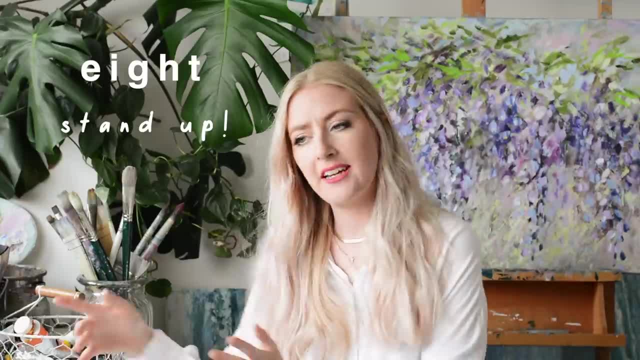 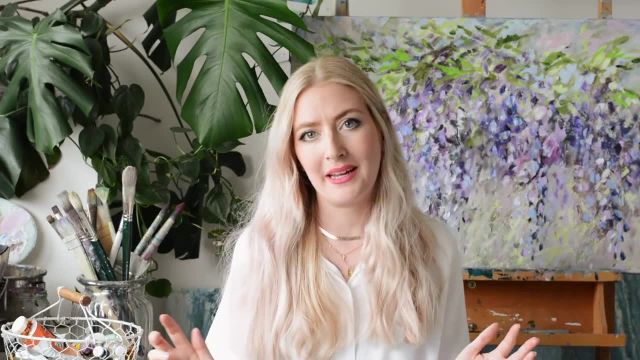 often we can sit down, but actually standing up means that you have more freedom. sorry to hurt yourself, Standing up allows you to have more freedom as you're moving around your painting. It can help you be more free-flowing. get the music on, get that energy up. That can. 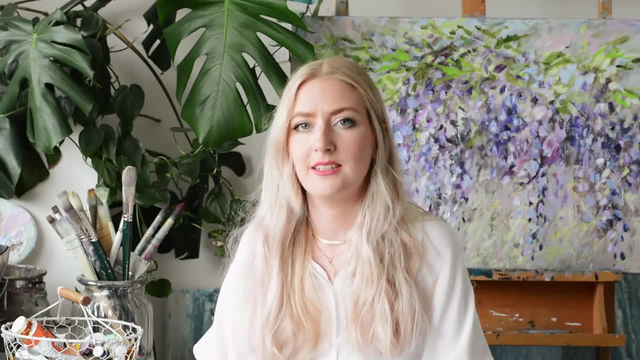 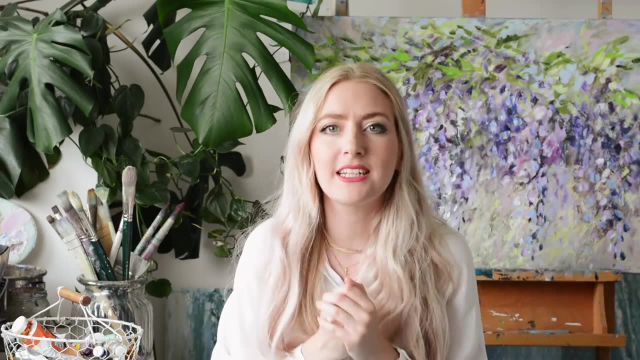 really help. you just input some of that blah into your painting and dab a big blodge of paint there and dab a blodge of paint here and grab some of that and grab some of this and that can really just help your painting like come alive in itself and have its own story. Tip number nine is to train. 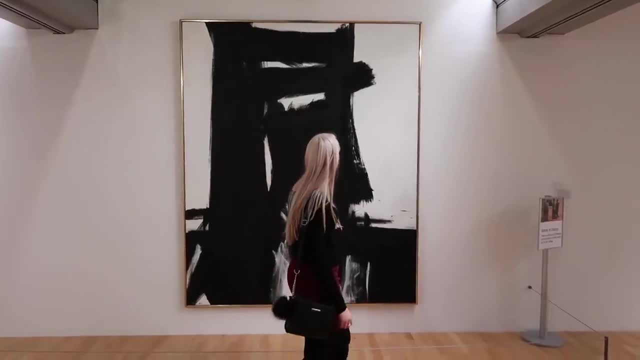 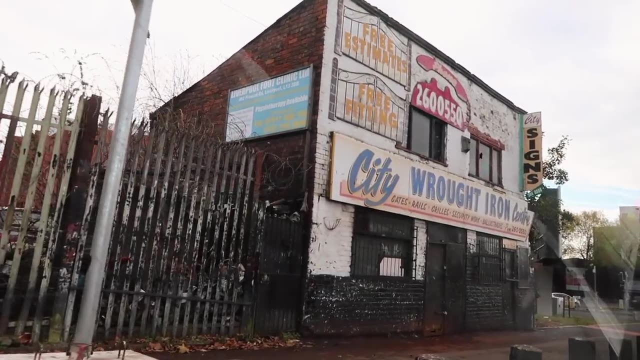 your eye to look at things in an impressionistic way. So this involves looking at the world differently, and this is great, especially if you're an artist. that doesn't have much time, because you can do this anytime. You can do it while you're working, while you're going for a walk with the 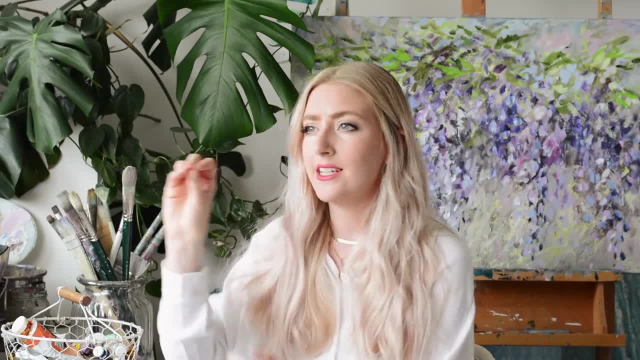 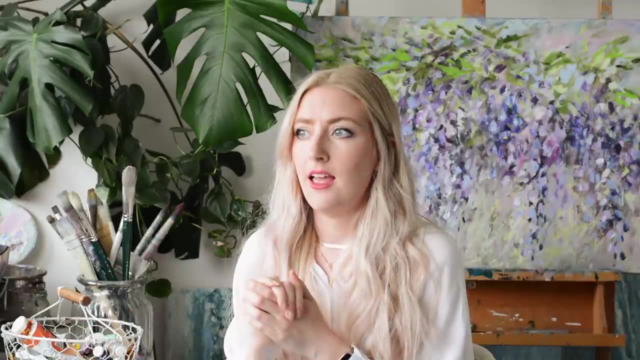 dog, When you're looking out at something, think what is the value in that, Like, how bright is that? It looks green, but is it green? Is it a dark green? Is it a light green? Is it a blue green? Is it a? 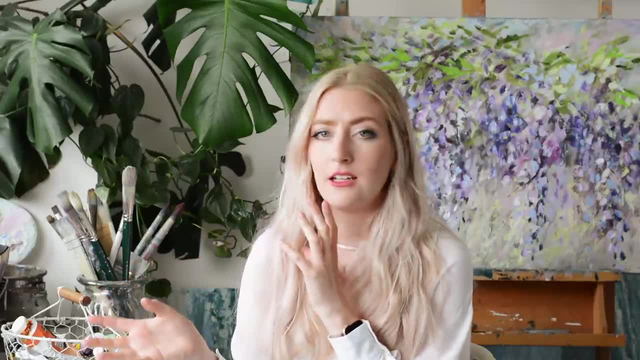 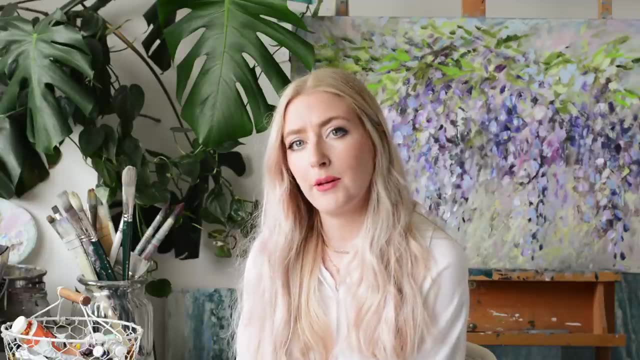 yellow, green And train your eye to see things in a totally different way. So instead of looking at that, instead of it just being what it is, you can pick up little things that could help you in your painting. I don't know if any of you guys were like this, but when I really started getting serious- 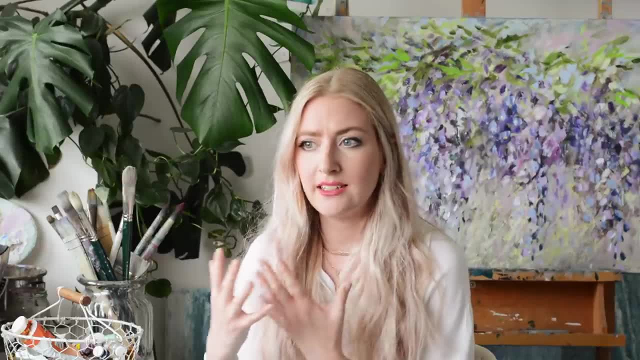 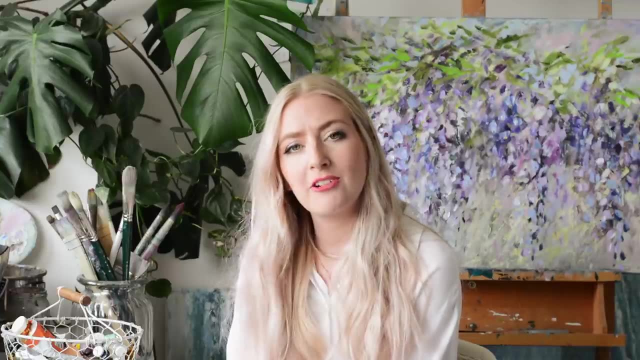 about painting an art. it was like I couldn't help myself. Like as I was talking to people I'd be thinking, hmm, how do I paint that eye? or oh, the shadow here? that's just capturing. it's very green. I'd add a bit of green if I was painting them. So I don't know what my face was doing when I was. 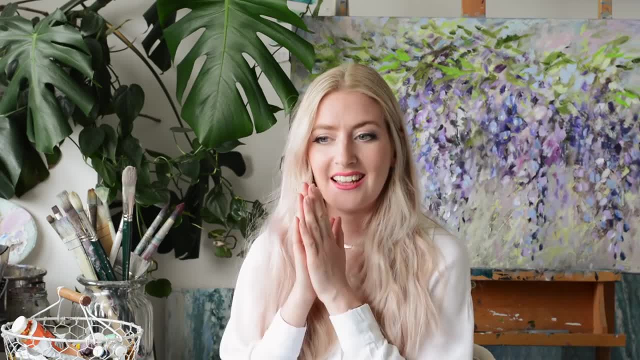 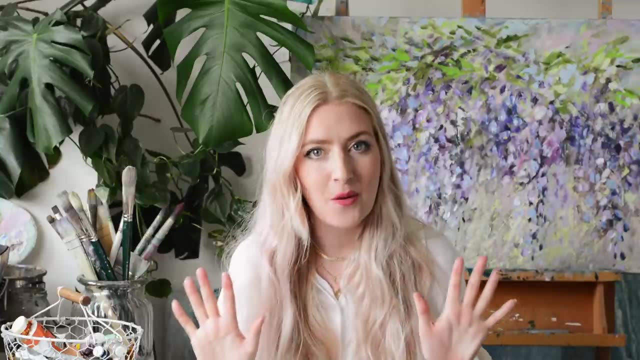 looking at their face, but it's almost like you can't help yourself once you get in that sort of way of thinking, and that can really help when you're painting. Tip number 10, which I think is one of the best ones, is to give yourself a time limit. Working fast naturally means that. 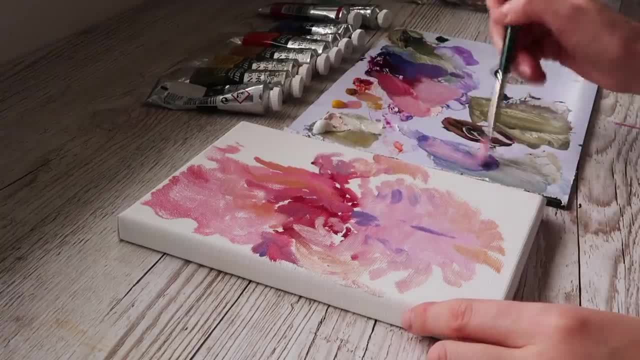 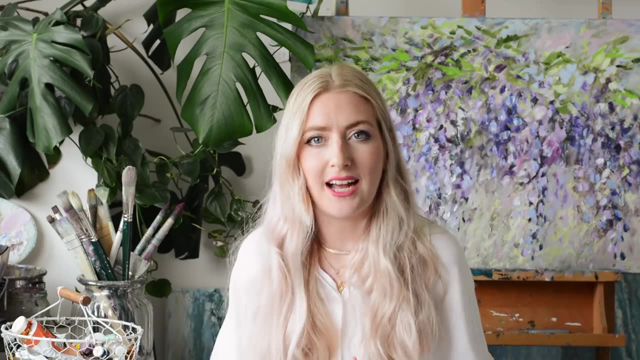 you have to paint in an impressionistic way because you're rushing and you can't get all the details. So set yourself a 10 minute timer, 5 minute timer or 20 minute timer and work fast. Work like you've got a purpose and, like you know, you've got a timer on and that can really change. 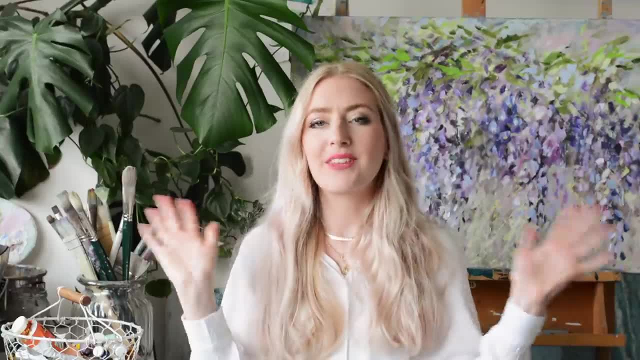 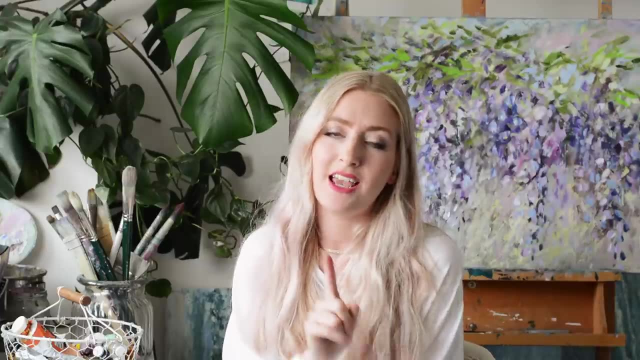 how you work and change your practice up. So there we go. there we have it: 10 tips to help you paint in an impressionistic way. I really hope that you enjoyed them. let me know in the comments what your favorite tip was or if you have any other tips for everybody and that will be really helpful to. 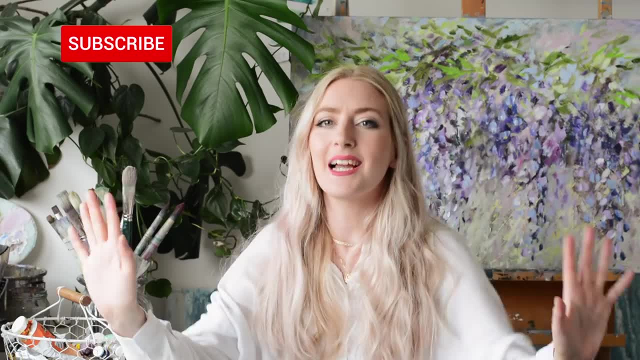 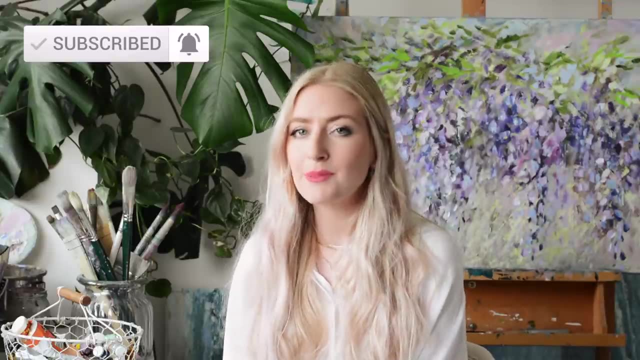 everybody watching. If you enjoyed the video, please, please hit the like button. subscribe. hit the notification bell so that you don't miss future videos. Go and check out my painting tips and tricks playlist for more tips on all sorts of painting tips and tricks. I'll see you in the next video. Bye for now. Subtitles by the Amaraorg community.